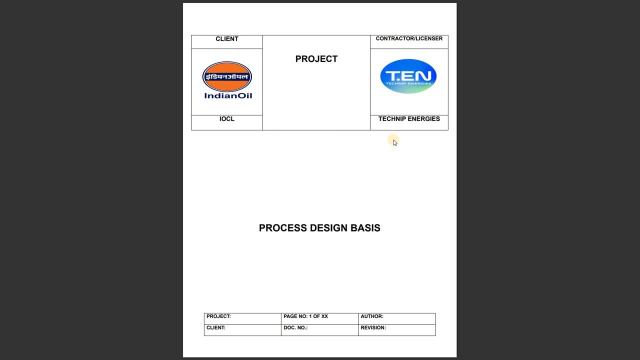 okay. There are other companies as well, like McDormand, Flo, Daniel, Saipem, etc. And there is the client. that is IOCL Means the client is IOCL. Okay Means you are preparing the process design basis for the IOCL. and the contractor or licensor is the Technip, Means the BDEP. which who is 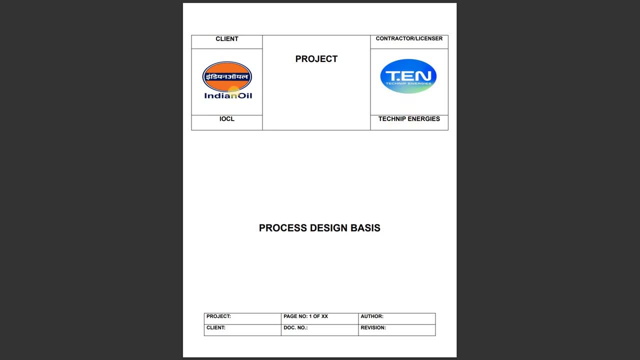 preparing the BDEP. Technip is preparing the BDEP. Okay, For IOCL, Are you getting my point? And there are other companies mentioned here? Okay, Let's suppose that that product, that project could be about the refinery. Okay, That project could be for a particular plant, That could be a DM plant. 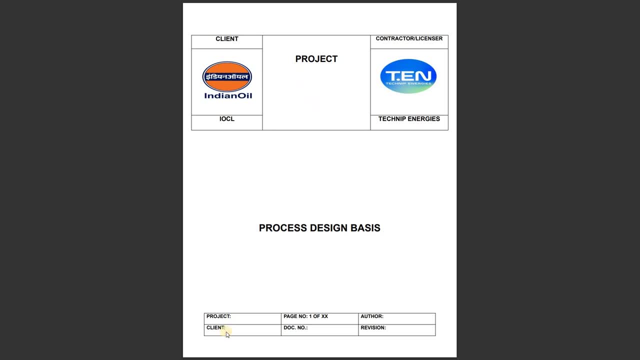 That could be any other plant. Are you getting my point? What I want, what I want to say, Then, in the footer you will like, you will mention about the project, That could be the number, basically about the client. You will mention here the page number. It could be one of, let's suppose, 50,. 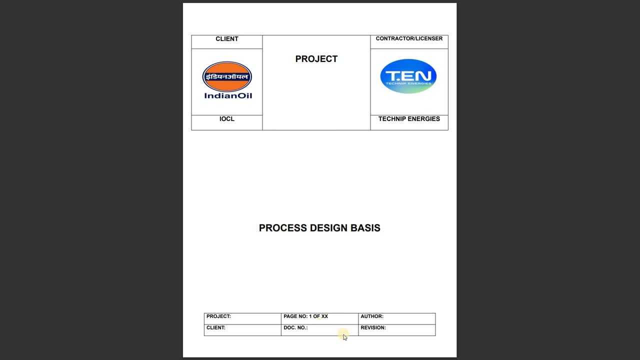 100, anything else, The document number you will mention here for your reference. Who is the author and what is the revision you are mentioning here? Okay, So that you will mention. I hope you understood about the cover page, So now just understand that- what information we provide. 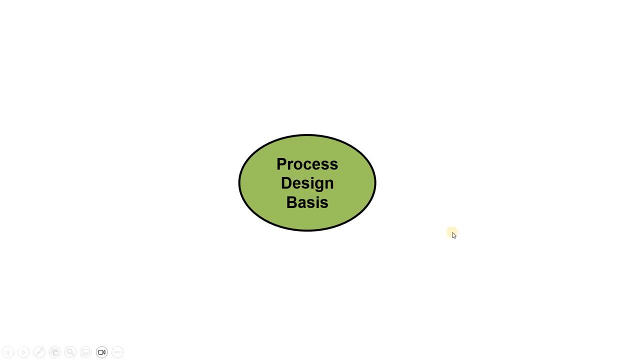 in the process design basis. Okay, So this is very, very important for you And I'll I'll simply say you: please watch this video carefully, because this video is going to be very, very helpful for you if you are a fresher. So the first information: 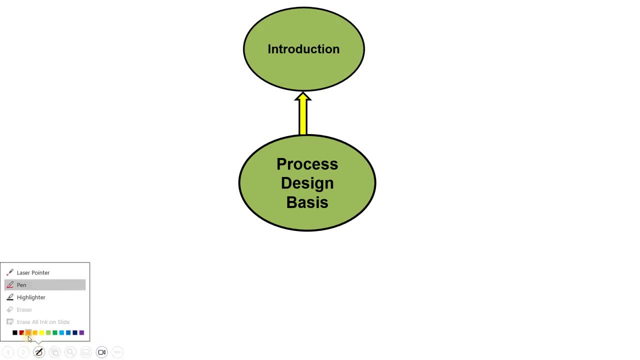 which we provide in the process design basis. that is the introduction. You will give the information about the your project. Okay, What is your project? What is the background of your project? That information you will provide in the introduction means who is your client? which? 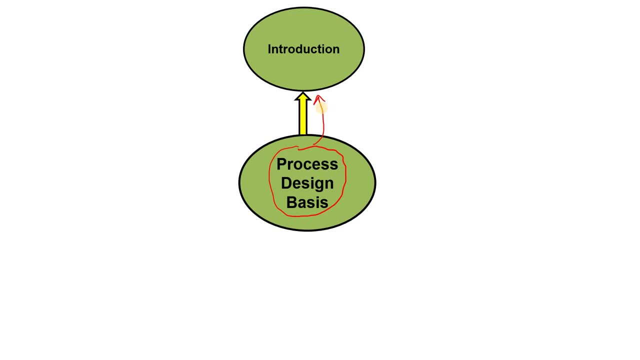 what is the location of your client? Okay, Let's suppose it could be within India, It could be outside India, Okay, So geographical location. simply, you will write here. Okay, What is the capacity of the plant? Okay, That you are. 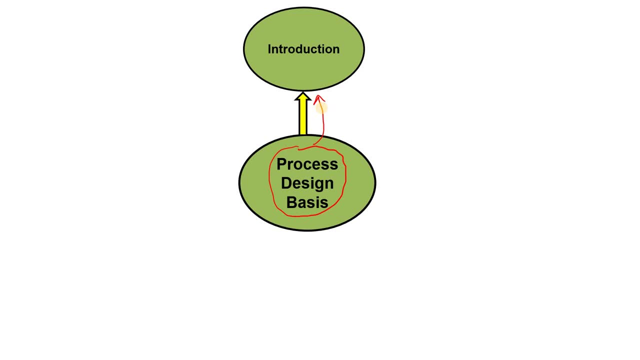 you mentioned that you will mention in the introduction, or whether you are doing the engineering or procurement or commissioning That you will mention in the introduction. I hope you got my point. Then the next information which you give in the process design basis, that is: 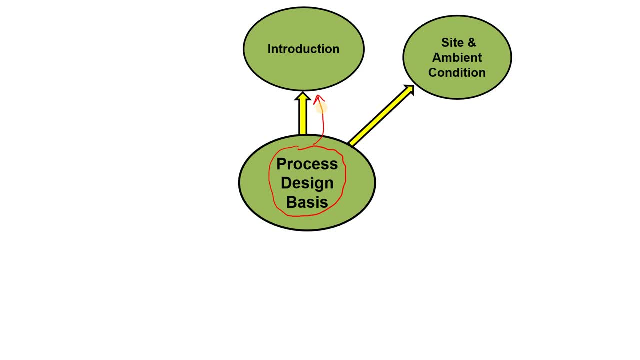 site and ambient condition, Okay. So why this information is important? this information- Okay, That is, site and ambient condition- is provided by the client. that information is here, Okay, provided by the client in the kick-off meeting or after the kick-off meeting. okay, why this? 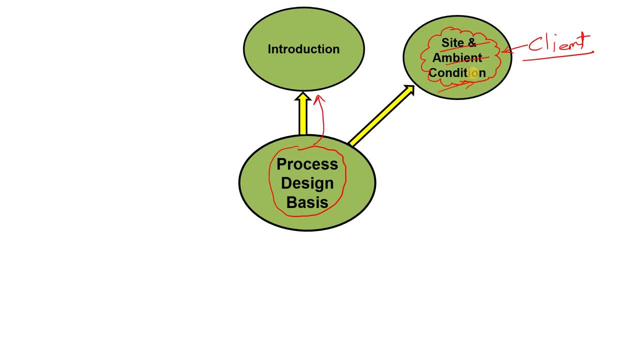 information is important- site and ambient condition- because, on the basis of this condition- okay, the information which is provided in the site and ambient condition- you do the design. okay, like you do the design of the cooling tower or chiller or your, if whatever the equipment which you are using where ambient condition could play a important role, their site and ambient condition. 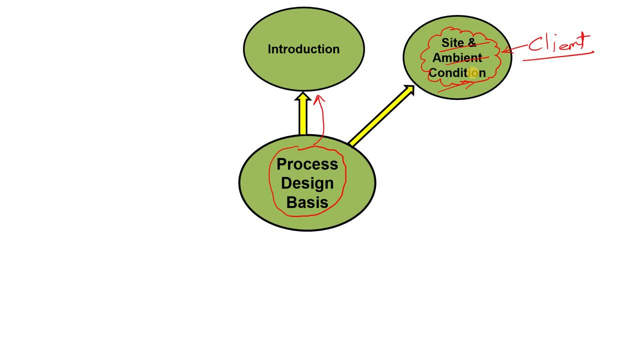 plays a very, very important role, for example, in the site and ambient condition. you will find out that you will get the information about the temperature. let's suppose if your client plant is in the, let's suppose, in the europe, in the europe your client plant is okay and there is. 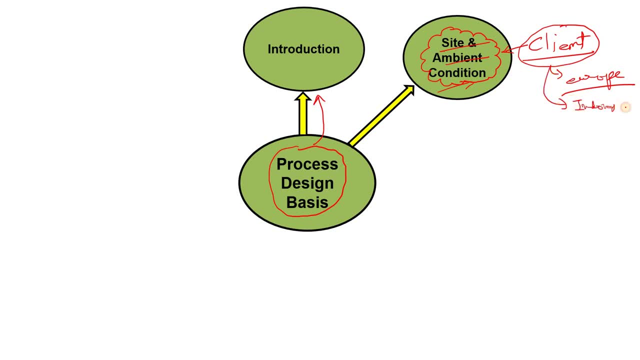 another client whose plant is in indonesia, and there is the third client which plant is in australia. okay, so the site and ambient condition is going to change, means minimum and maximum temperature is going to change, wet bulb temperature is going to change, wind speed is going to change right, and also the electric power means voltage. 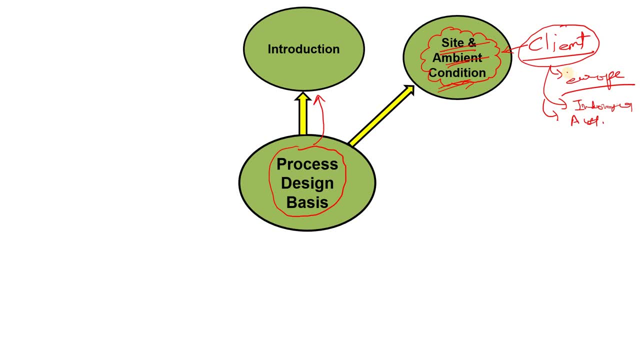 is also going to change. are you getting my point? what i want to say? so it will affect in the designing, whenever you will design the, your heat exchanger, your cooling tower or chiller, or chiller. and there is the third client: which plant is in australia? 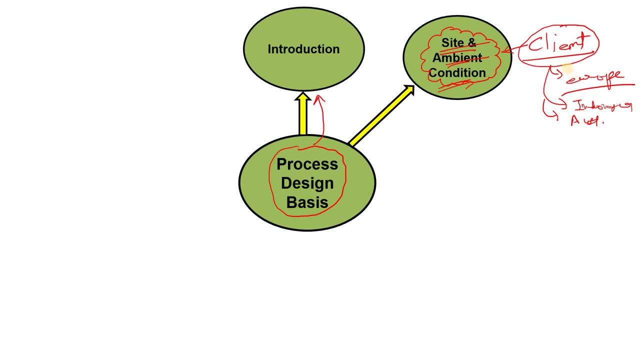 cooling tower, your chiller or any other equipment which you are going to design, so that design will be affected. that's why what we do, we ask client to provide the site and ambient conditions. this document is provided by the client and which which we mention in the process design basis. i hope this. 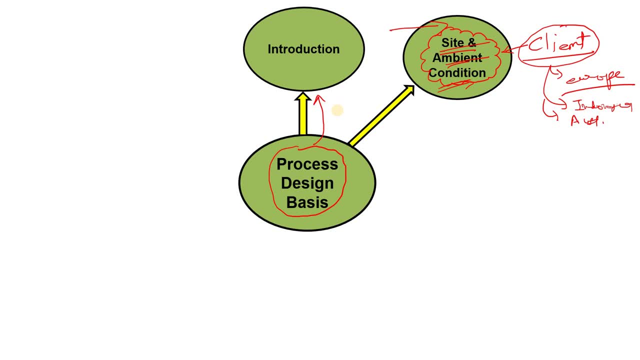 point is clear to you now. the next information which we provide in the process design basis, that is, that is your process description. that is your process description. okay, so what is what we provide in the process description? so basically, how your plant means, in which principle your plant is going to run, what are? the section is: 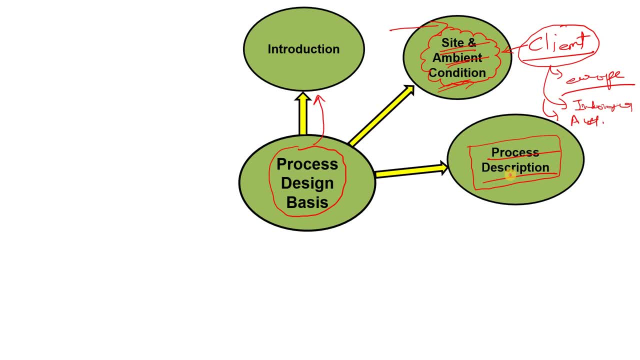 there. that mainly we provide in the process description means you will. so briefly, you will describe the, your process. okay, let's suppose if you are doing the one bd ep for the for the urea plant, for example, for the urea plant, you will give the process description, like how this urea will be manufactured. okay, how this urea. 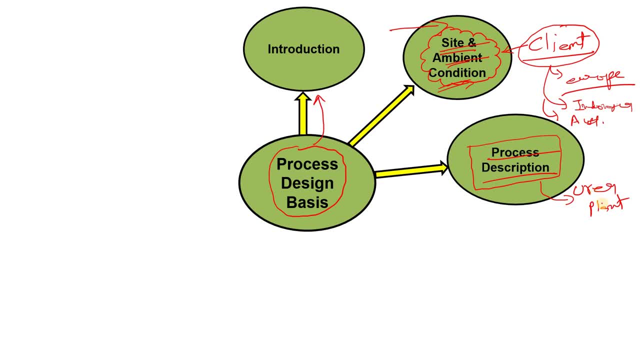 will become the urea from the raw material. what are the raw material for the urea? that is, carbon dioxide and liquid ammonia. okay, so how you will describe that? first of all, you will describe that this urea plant is based on xyz technology. that could be toyota. that could be sanamprogate- okay. 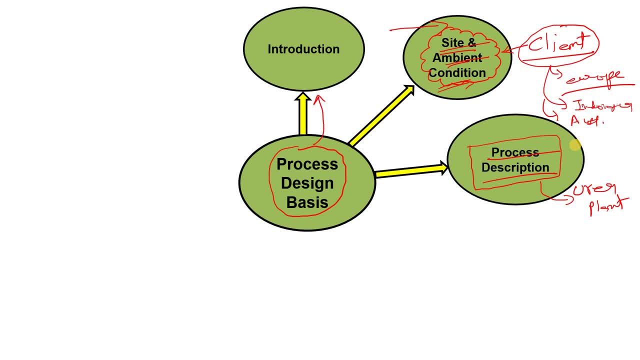 let's suppose if we take the example of the sanamprogate, then you will also describe that. there is the first of all there is the reactor. okay, in reactor the liquid ammonia is coming from ammonia receiver tank and the carbon dioxide is coming from the compressor section. and after that, 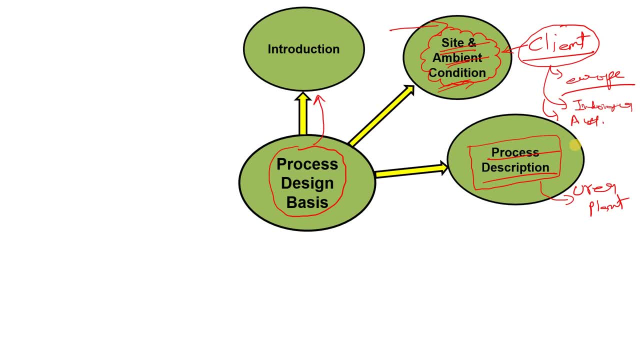 is: it goes for the decomposition, and after the decomposition it goes for the simple concentration, okay, and after that it is goes for the cooling tower, right? so this is the process description for the urea plant. same will be for the sulfuric acid plant. what you are doing, first of all, you 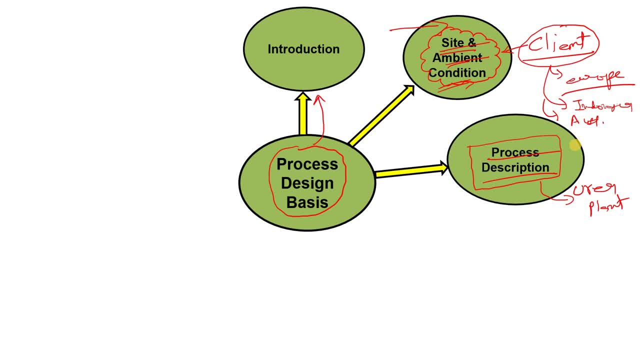 are melting the sulfur, then you are sending it to the burner, then, via sulfur filter, you are sending it to the burner. after the burner it is going the converter, then in the absorption towers and drying towers, and after that it will go into the your storage section. are you getting my point? what i want to say? so that is. 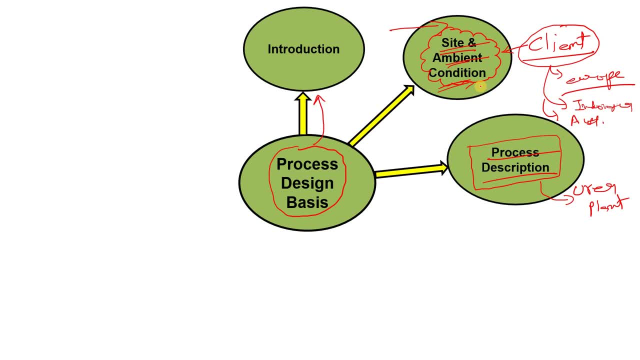 that is the process description. okay, so about the each document we are going to discuss in detail, okay, so if you want the video about the each topic, like what is the process description, what we consider in the process description, so let me in the comments box so i'll prepare the individual video about the each topic right now. the next information is: 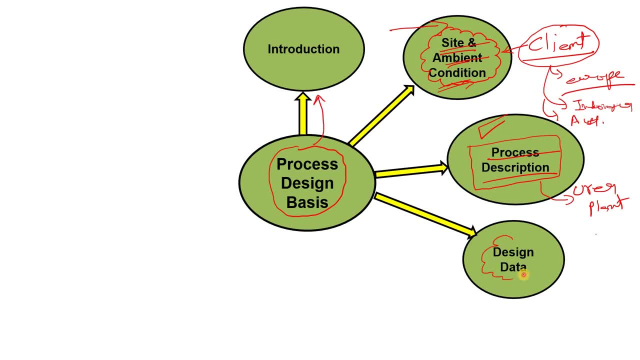 design data. so in the design data you will provide the information about the. what is the plant capacity right? what is the plant capacity of your project? what will be the turn down and up down range? what is the annual running hours? what? what will be the daily running hours are you getting? 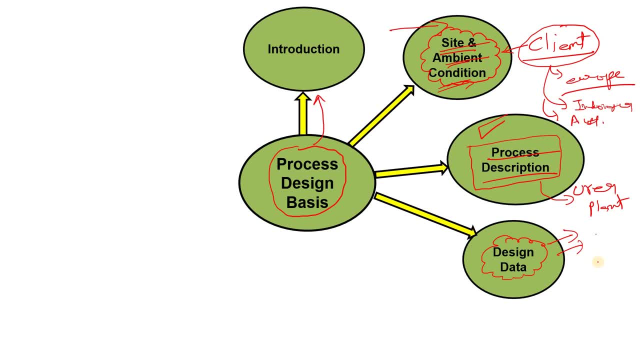 my point: what will be the concentration of your raw materials? if there is the gas or anything, what will be the purity? simply, you could say what will be the conversion, what will be the efficiency that you are going to discuss, or in the that you are going to give the information in the design. 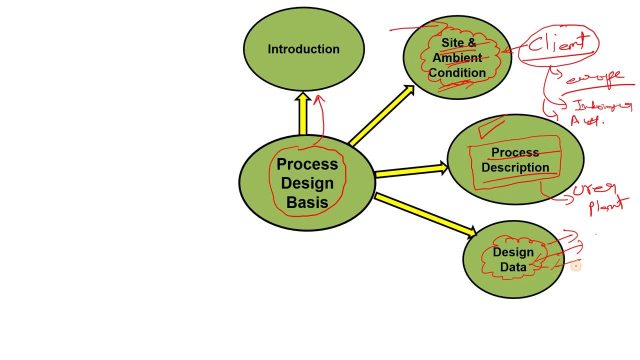 data section. there are the other information also we provide about the like: what is the end product, and that all that we also provide in the product specification. then the next information we give about the product specification: so so what will be your end product like if there is? the end product is urea, let's suppose if there. 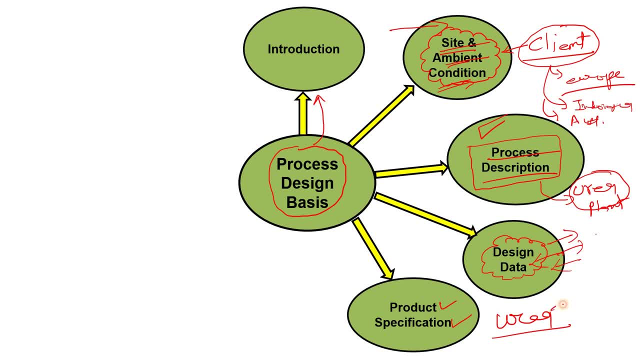 is the end product is urea. now, what information you will provide in the urea? you will provide that. what is the concentration of that urea? so let's suppose, if it is the 99.9 percent, then you will give the information about the. what is the free ammonia? is there? what is the? 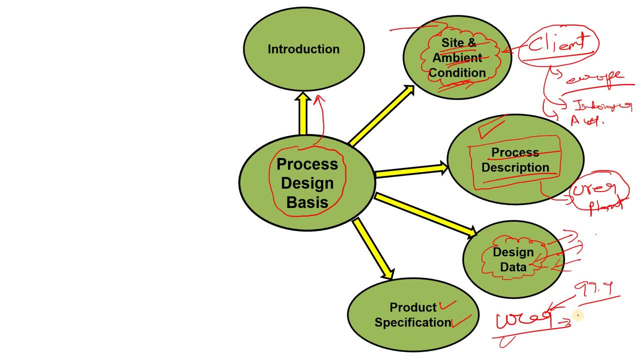 moisture is here right. so in the end product, what you will give to the client means you are giving here, you are giving the surety to the client that in the end, if you will buy the like license from us, if you will, if we do the bdp for your project or if we do the epc for your project, so we will. 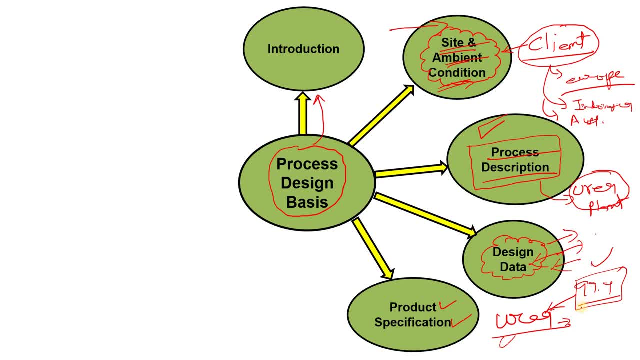 or we will provide you the debt efficiency or debt concentration of the product, that is, 99.9 percent urea or, let's suppose, 0.5 percent free ammonia, like that. are you getting my point? so that is the end result which you will provide to the client so that information is provided in the 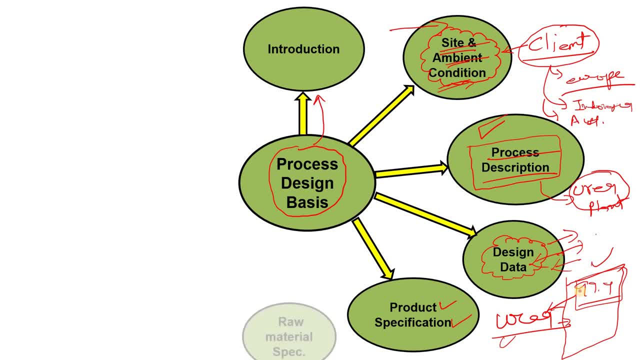 product specification section. i hope you got my point now. the next information is which we provide in the process design basis, that is, the raw material specification. okay, what is that? basically? it is, if you are manufacturing the urea, then what? what are the raw materials? so the raw materials are simply your liquid ammonia, that is, ns3, the 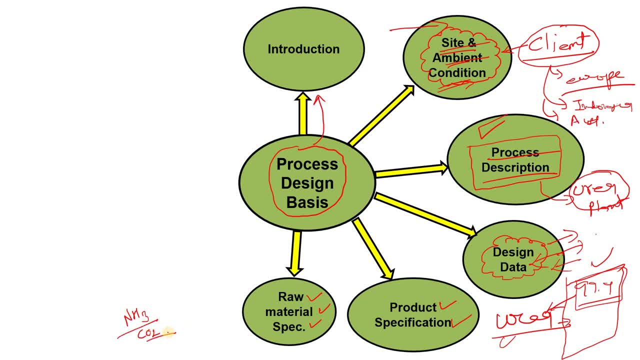 carbon dioxide. okay, and there is the steam and all that other information we will. we will give the. that detail in the utility specification mean, like liquid ammonia and carbon dioxide is your raw material for the urea manufacturing, right? so you will provide the information about the ns3, and carbon dioxide means what is the purity of the ns3, what is the pressure? 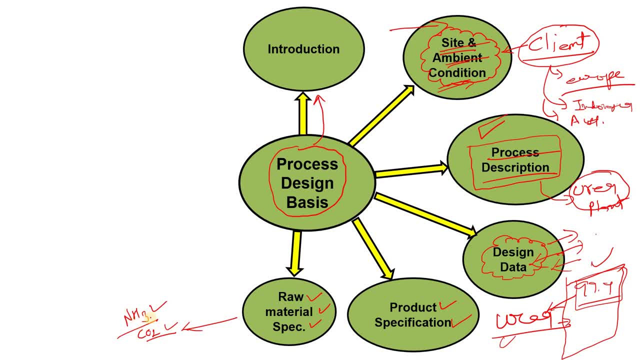 temperature? okay, and what are the other traces within the this, this ammonia, in in this carbon, carbon dioxide, that information you will provide in the raw material specification? let's suppose there could be the moisture, there could be the water vapors, there could be the other traces of. 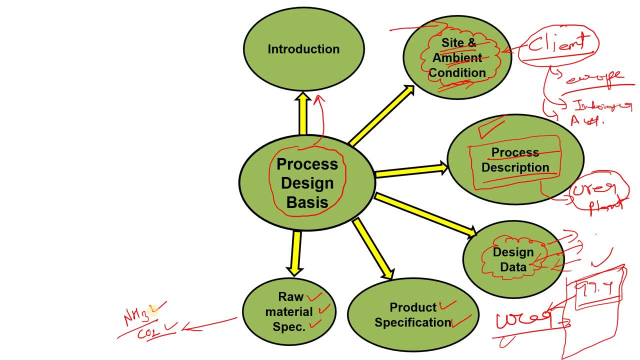 the like composition. like it could be hydrogen. it could be any other composition of the gases as well. okay, so that you will mention here- because this is the, what raw material we are going to use to manufacture the our product. okay, this information is very, very important while designing. 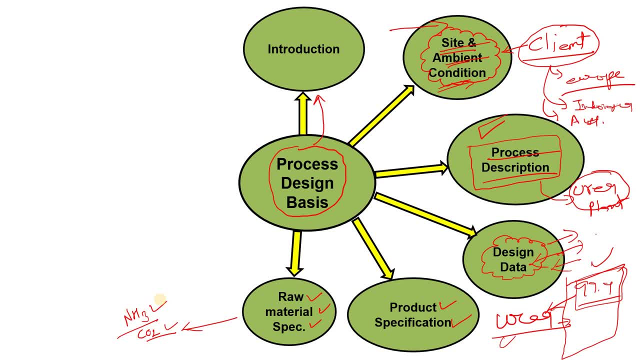 the plant. then the next information which we provide in the process design basis, that is, your chemical and consumables specification. okay, so i just remove here this one. okay, what are the chemicals you are going to use and what is their consumption? that information we provide in the 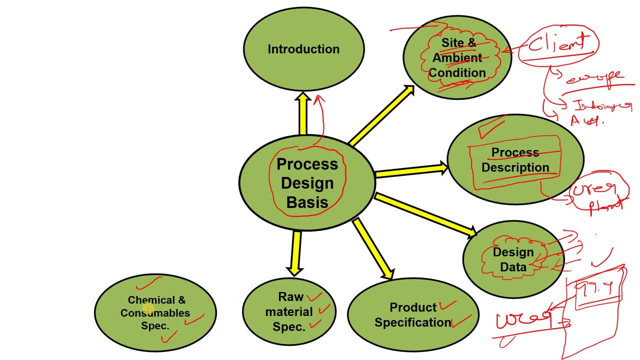 chemicals and consumables specification. so if the chemicals, if there is some chemicals if you are that could be your catalyst, that could be your any other chemicals, okay, that you are using as an additive, so that information also you will provide here that could be activated alumina, that could be like vanadium pentaoxide, that could be any other right so that. 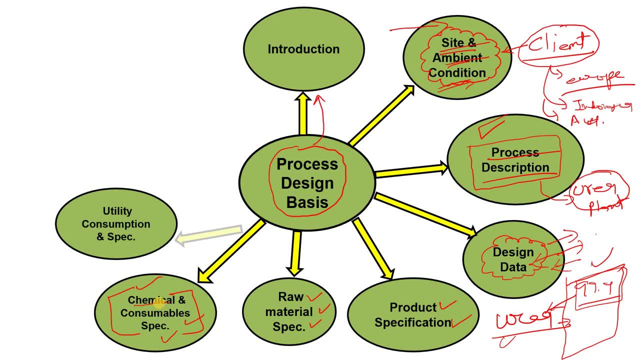 information you will provide in this section. now. the next information is: we provide about the utility. okay, whatever the utility you are using, like utility, consumption and specification section- we provide where we give the information about the utility. okay, in the utility, what is comes in the utility, that could be your dm water, that could be your process water, raw water, that. 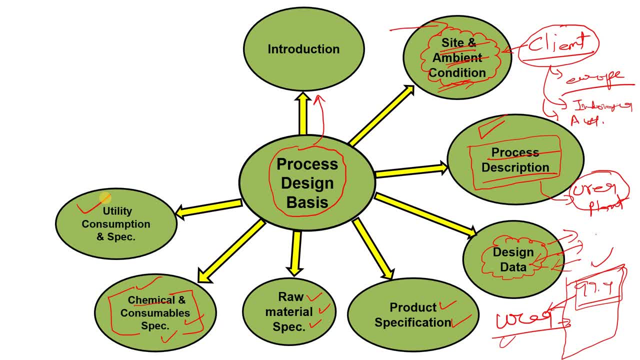 could be your steam, that could be your high pressure steam, low pressure steam, medium pressure steam, that could be your nitrogen instrument, your plant here, so that all information you provide in the utility, consumption and specification section okay, what you will provide here, you mean you will provide here the quality, for example, if the process water is coming from the client. let's suppose 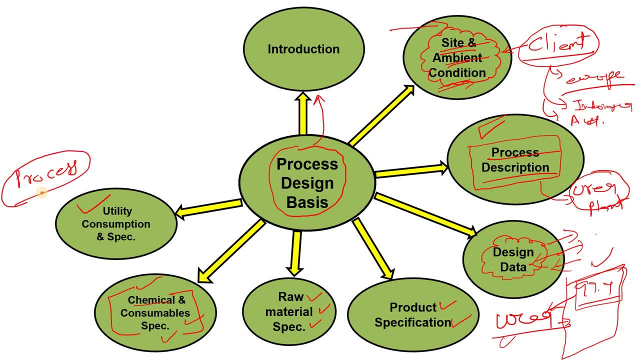 so he will send you the one result, the process, like, whatever the process water he will provide you. he will, if he will provide you any process water. so what is its tds, what will be its ph, what will be its hardness, pressure, temperature. that all information is provided by in the process water seat: right same, if you are. 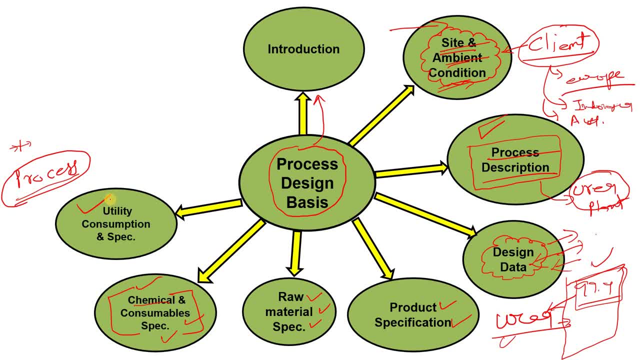 like, let's suppose, if you are mentioning here the dm water, so what is the precedent temperature you will mention here, what will be? if you are mentioning about the cooling water, so what is the outgoing temperature of the cooling tower, of the cooling water to the cooling tower, what will be the 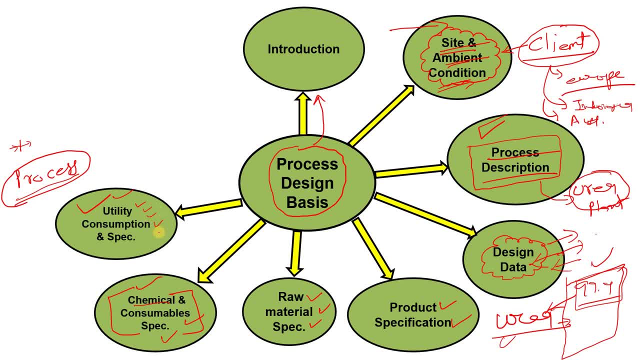 wet bulb temperature. what is the nito if you are using the nitrogen? so at which temperature pressure you are? you are using the nitrogen in the plant, okay. what is the purity of that nitrogen, so that all information is provided in the utility and consumption specification? i hope you are getting. 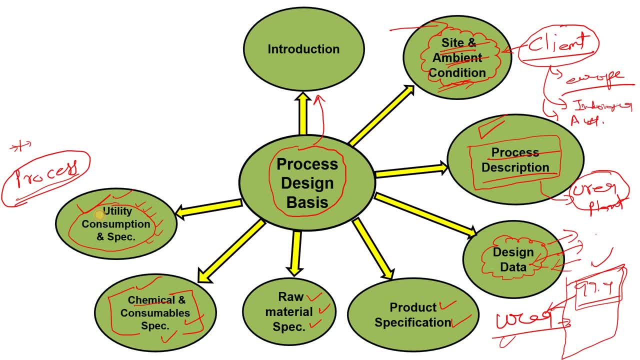 the point same. if you want to know about the in detail, about the each section, so you could simply share in the comments box. so i will prepare the individual video about the each section. now in the, in the like last, we prepare about the one section about the storage facilities. 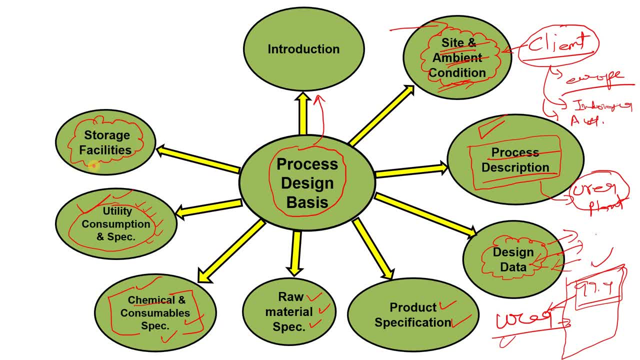 in the storage and facility section what we provide. we provide that we have manufactured our product, so where this product will be stored, there will be some tank, okay. there will be some division where we will store this product, okay. so that that storage facilities information we will provide in the storage facilities section are. 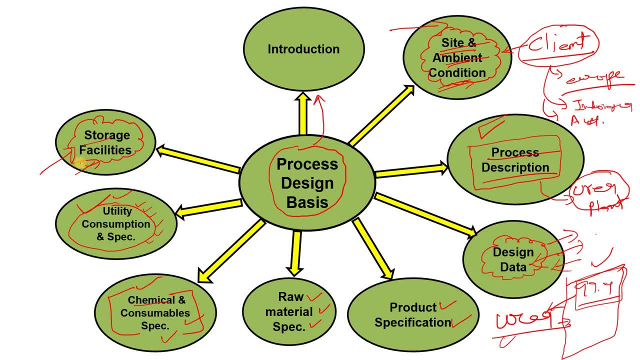 you getting my point? what am i saying? okay, let's suppose if you are storing the ammonia, so in the ammonia there is a storage tanks for that. storage tanks are double layer type. okay, that we will also discuss later. okay, in our videos. but what am i telling you? wherever you are storing the product, 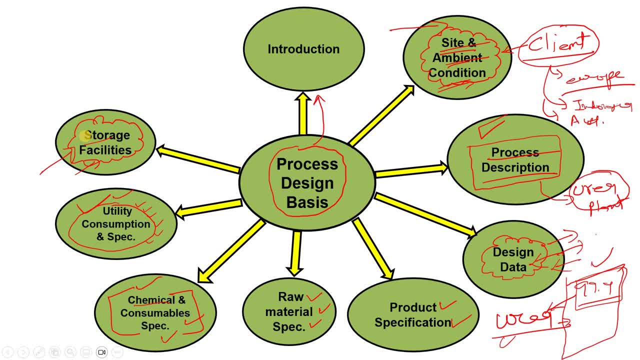 so you will, you will give the information about that, right. and in the last, we we give the information about the design codes and standard. what is that actually? this information is provided because, like, if we are designing the tanks, okay, so at which standard we are going to design that?